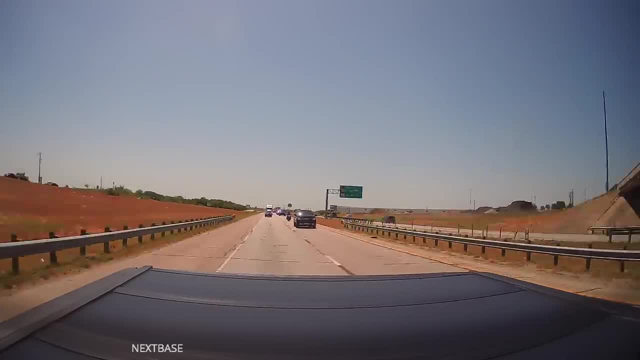 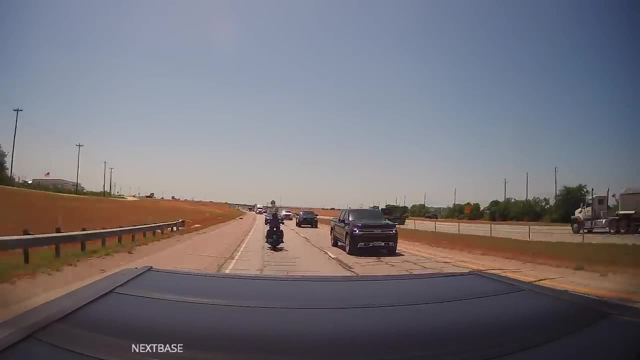 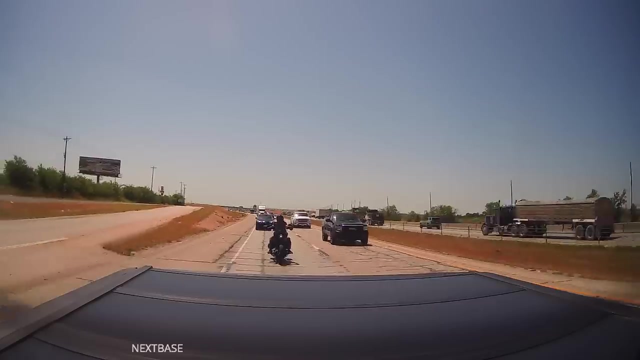 things up a little bit, We'll get to the point where he passes my truck. Notice the following distance that the rider gets behind my truck and his position on the highway. So we've got the entrance ramp to the left of the screen and our rider is going to use that to pass my truck on. 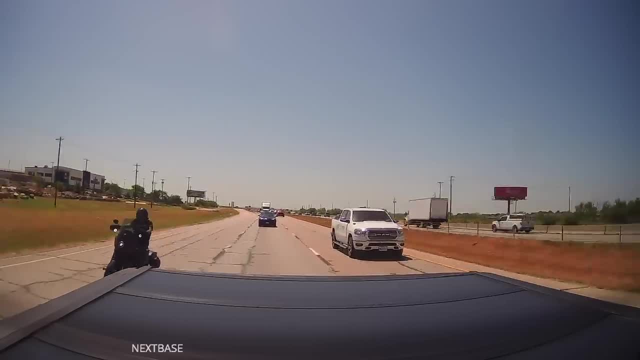 the highway. We'll give him the benefit of the doubt. So we're going to go ahead and get to the point where he passes my truck. Notice the following distance that the rider gets behind my truck. Maybe he thought the highway was adding extra lane, I don't know, But you can see how the 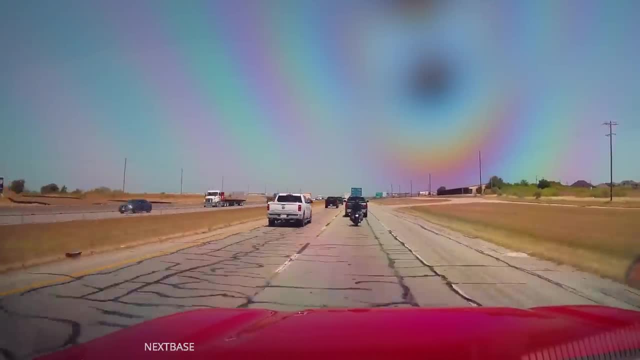 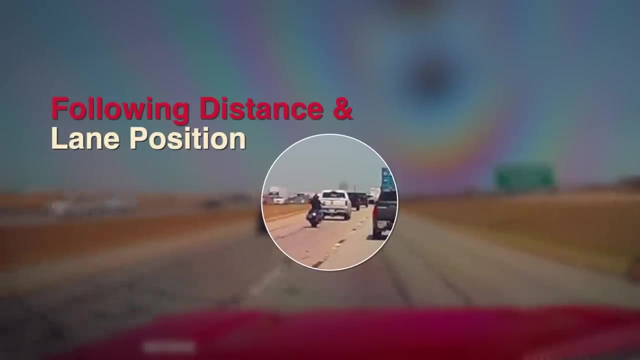 rider exchanges poor lane position and bad following distance to me to the truck in front of me, And then he moves to the left and continues his bad habit with the white truck in the far left lane. Some of you are watching this, thinking I don't see what the big deal is. The rider's just 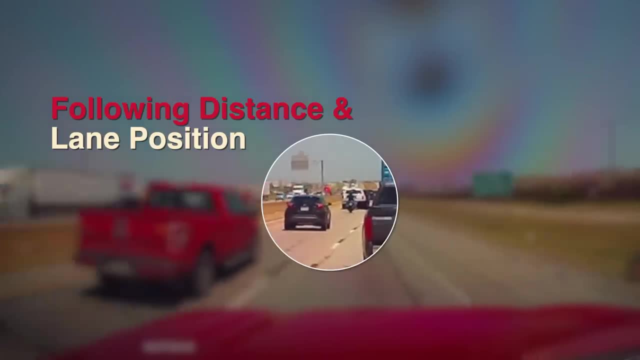 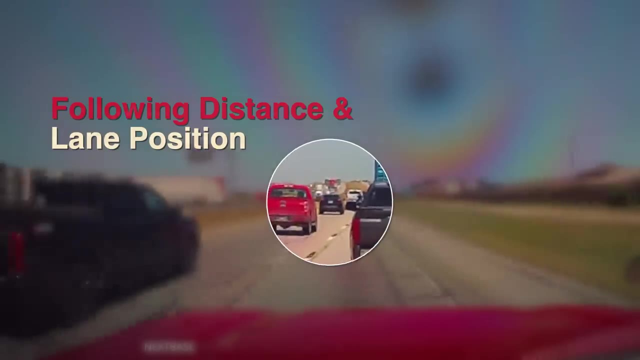 getting up the highway. I can promise you this: If you do not see the deficiencies in this rider's road strategy, your road strategy is going to be bad. So I'm going to give you a little bit of time to think about this. I'm going to give you a little bit of time to think about this, So let's. 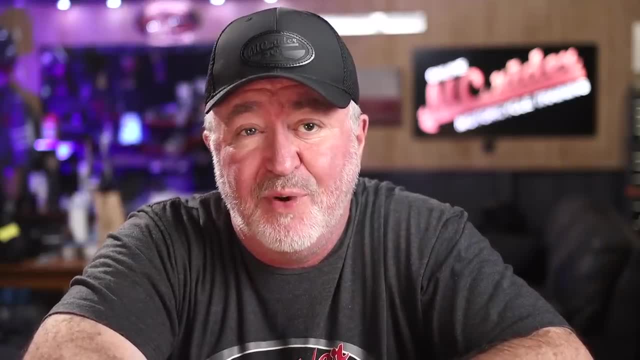 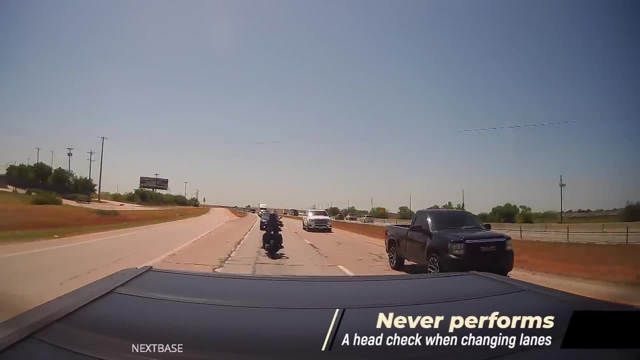 talk about a few things that we can learn from this rider and how we could decrease our risks out on the road. First of all, his following distance was really bad And I think if you watched MC Ryder for any length of time, you picked up on that right away In this video. 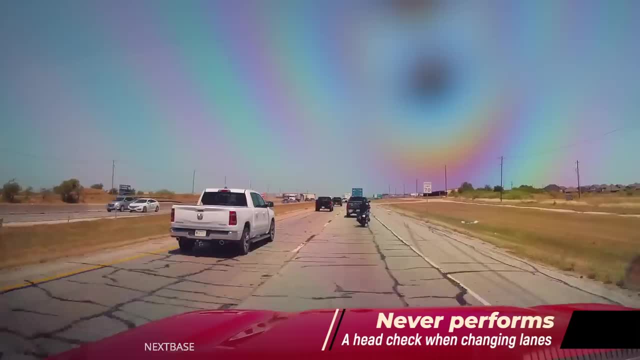 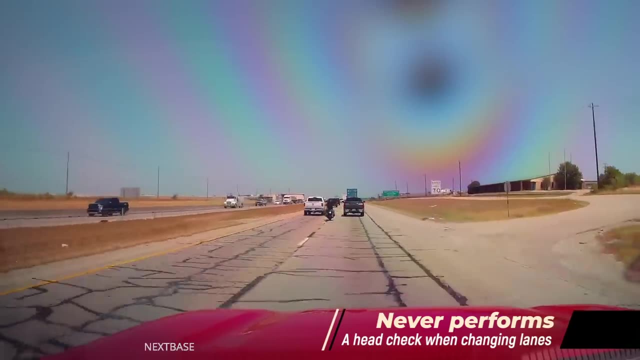 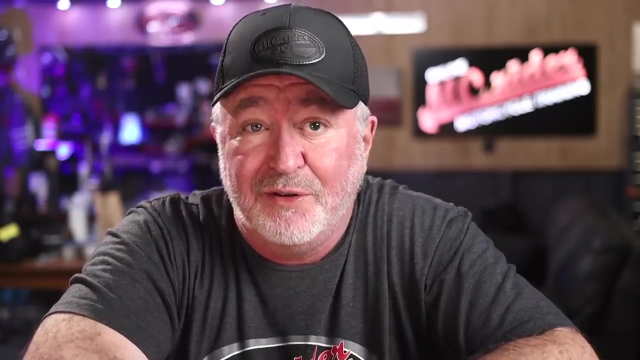 he consistently has less than a one second gap between him and the car in front of him, Initially behind me, then behind the Tundra, Toyota Tundra- then behind the pickup- he is consistently less than a second's following distance. To make matters worse, 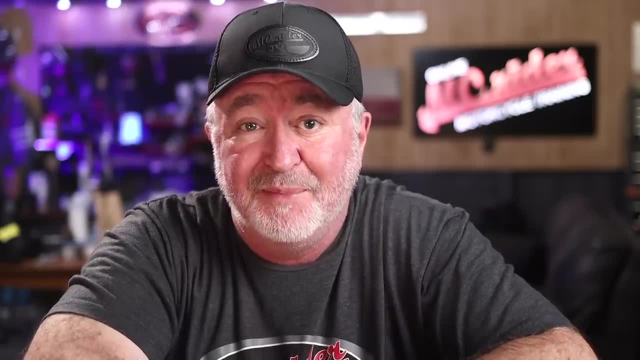 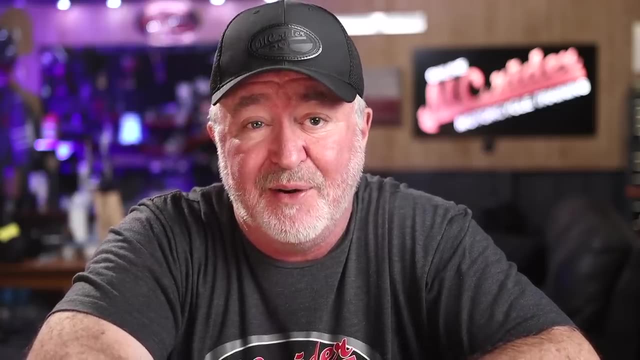 he's even doing this behind vehicles that make it impossible for him to see. So I drive a four-wheel drive Nissan Titan pickup. It doesn't have a lift on it or anything, but it still sits up much higher than this rider could see, especially being right on my tailgate. He moves from directly. 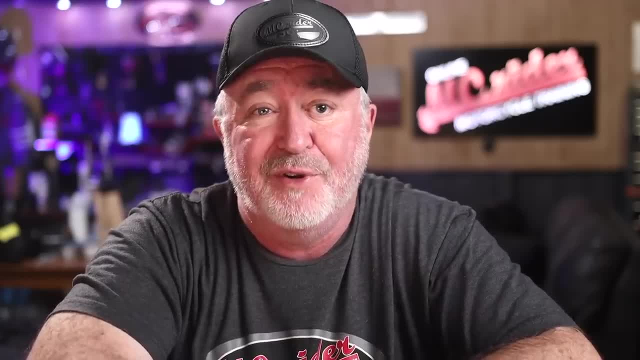 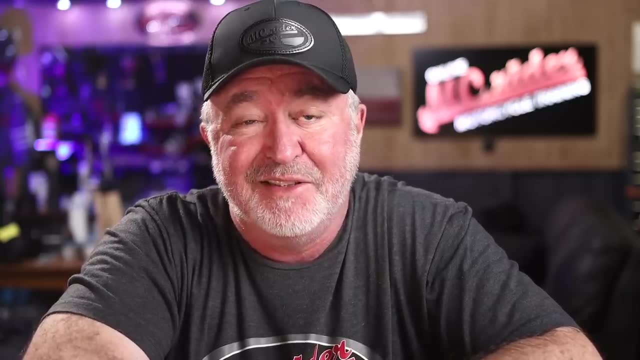 behind me to the bumper of a four-wheel drive. Toyota Tundra changes that out for the bumper of a four-wheel drive- Rambo. He's got a lot of room for improvement. He's got a lot of room for pickup. I guess it is true that Texans like their four-wheel drive pickups and this guy happened. 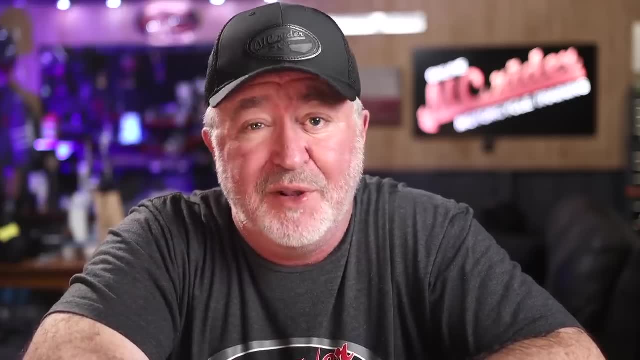 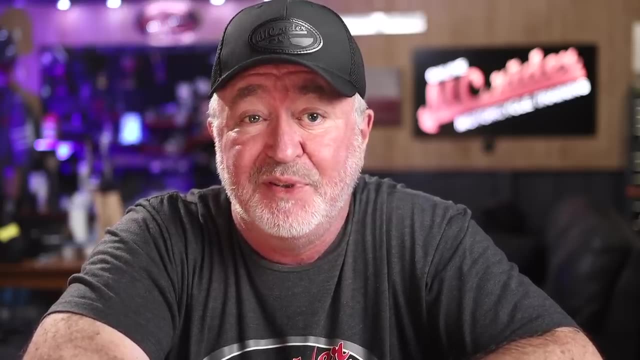 to find every one of them on the highway this day. So this Ryder is fully dependent on every driver in front of him to do the right thing, because he can't see what's happening up the road and he's positioned himself directly behind that vehicle in front of him so that he's got no reaction time. 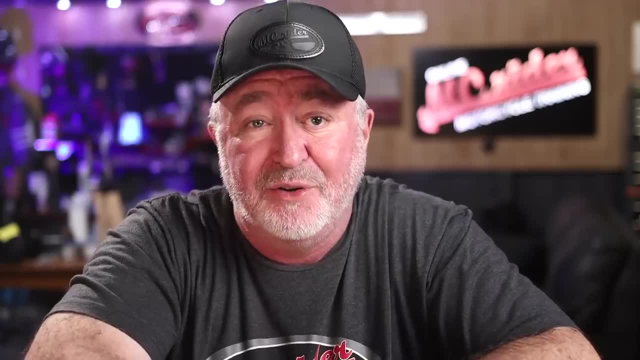 if he needs to change lanes or avoid a hazard in the road, Not to mention that he's attached to the bumper of trucks that can easily move him around. So he's got a lot of room for improvement. So he's got a lot of room for improvement. So he's got a lot of room for improvement. So he's got a lot of. 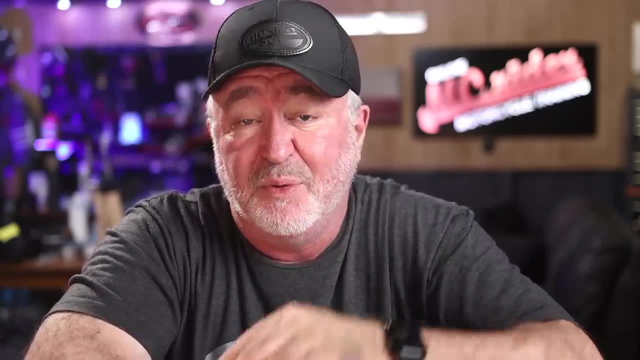 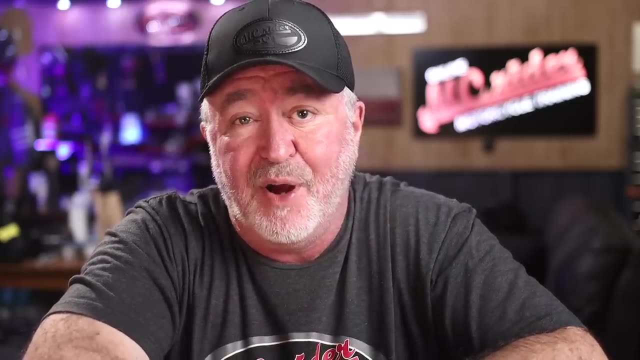 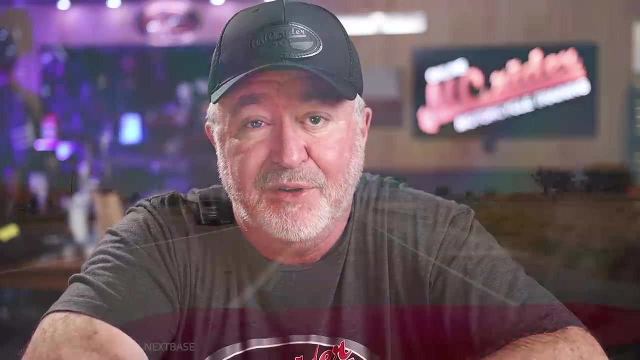 easily straddled debris that's often found in the road. So my truck sits up high enough that if there's a chunk of rubber I could just, you know, put it right between the tires and keep on going. You don't have that luxury on a motorcycle, And this was a hot day- It was about 104 degrees when. 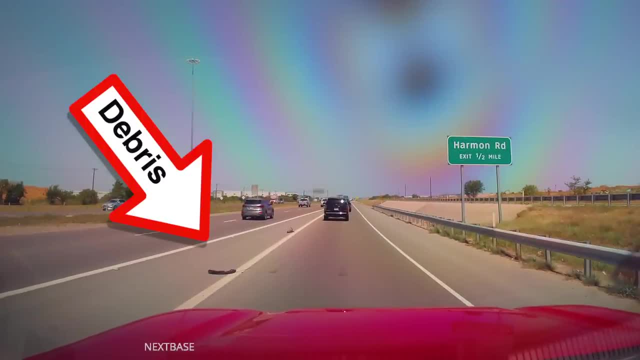 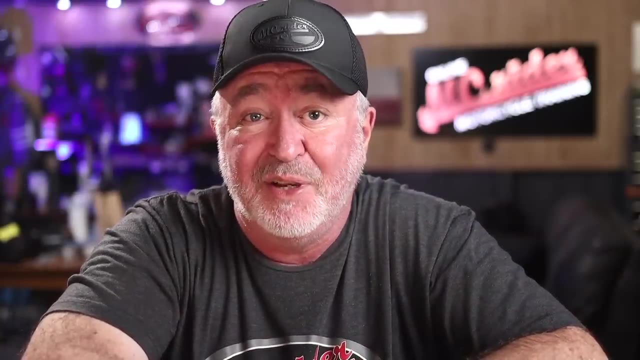 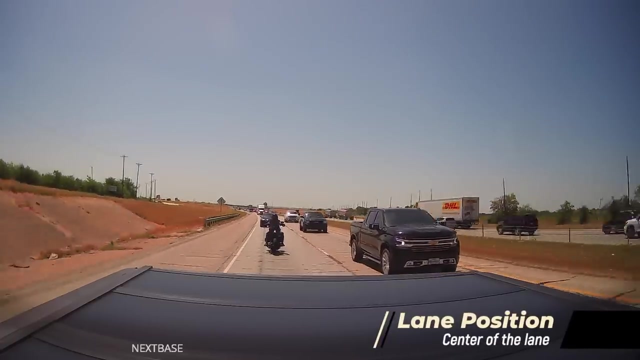 this guy was out riding, and 18-wheelers are losing rubber all over the road in temperatures like that, So it's not an unknown hazard by any means to see a piece of rubber laying in the road. But where he was positioned leads us to the second issue is not only was he danger close to the 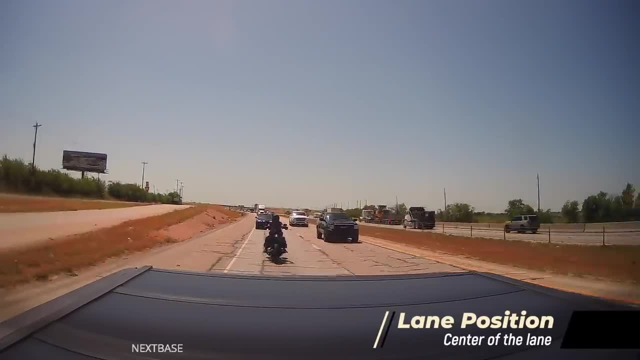 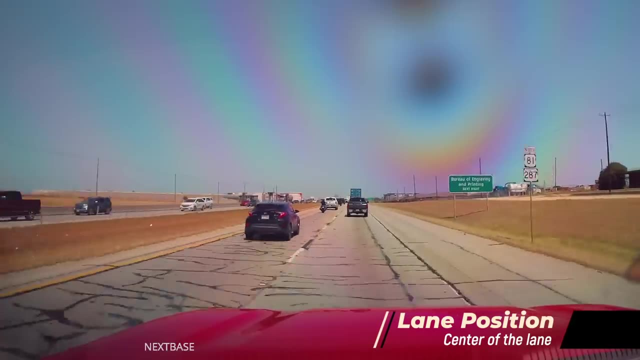 vehicle in front of him, but most often he was positioned directly in the center of the lane, directly in the center of that vehicle in front of him. This not only obstructs his view further up the road, but it increases his risk of hitting that debris, Even if he didn't increase his. 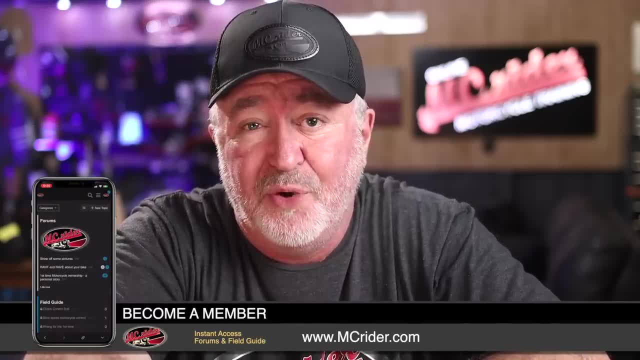 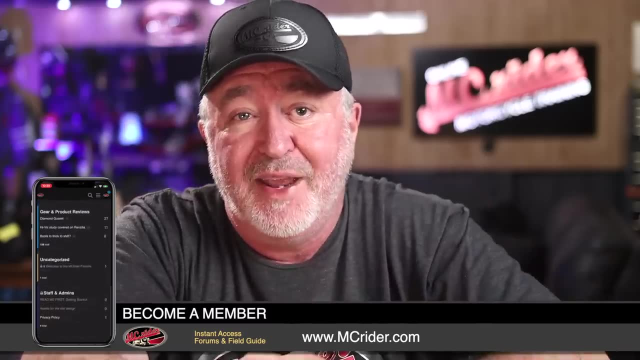 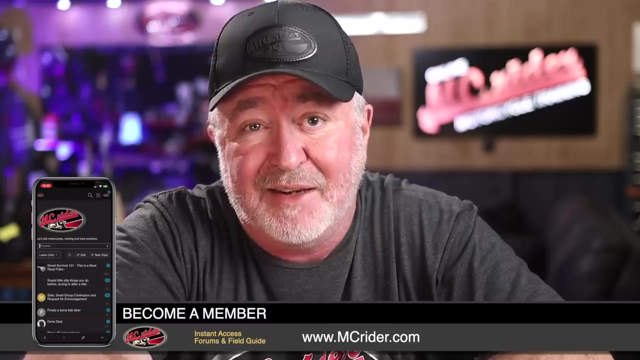 following distance and I can't think of a single reason why a rider wouldn't, especially in a congested city, position himself to the left or the right so that he could see past that vehicle in front of him. And, like I said earlier, I ended up being behind this rider to the same exact exit from 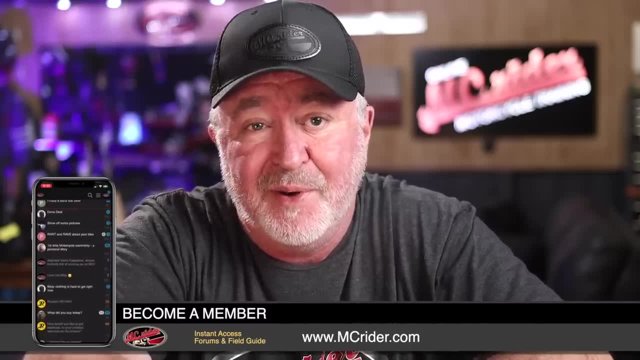 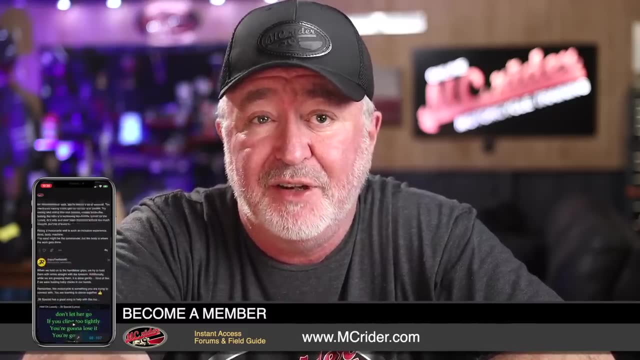 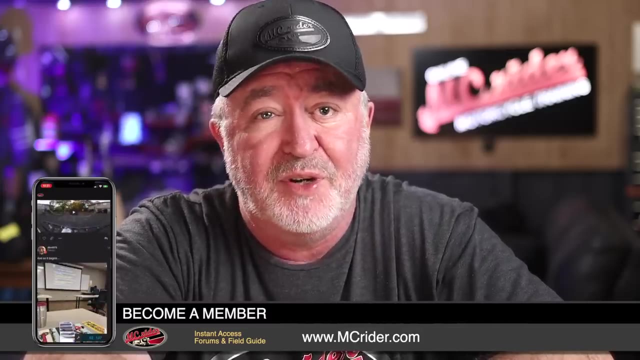 the freeway and he got there about 10 seconds in front of me. So he took all the risk and got no reward. Maintaining a proper following distance, especially in congested city, high-speed traffic like this, is a core road strategy. Any rider who ignores a simple two to three second following? 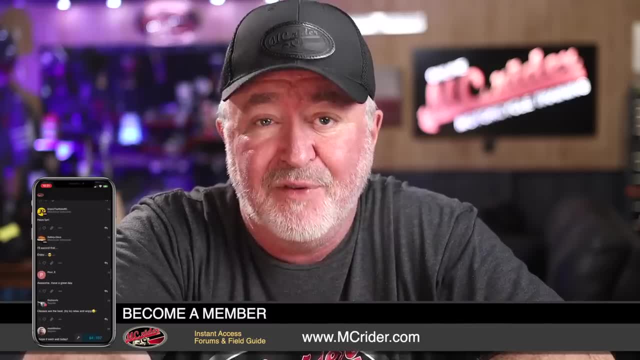